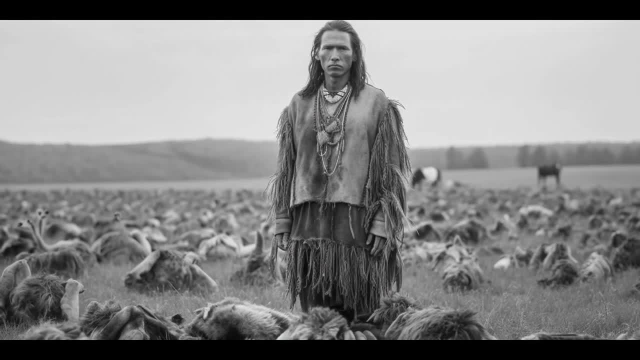 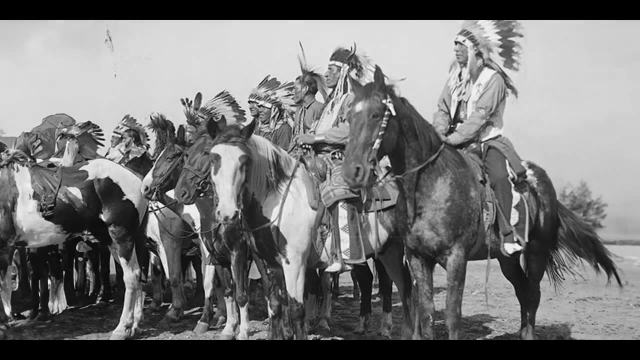 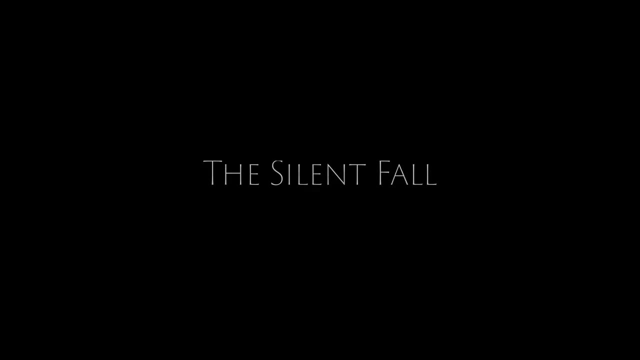 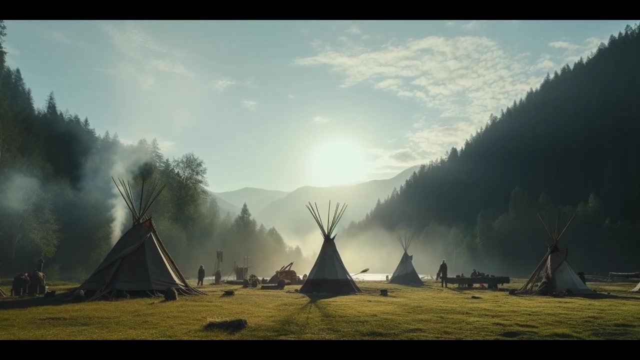 the lowest in history. More than a dozen tribes, such as the Pequot, Mohegan and Massachusetts, were completely wiped out. But what happened to them? What led to the near extinction of a whole race of people? In the early dawn of the 17th century, the untouched panorama of the New World became 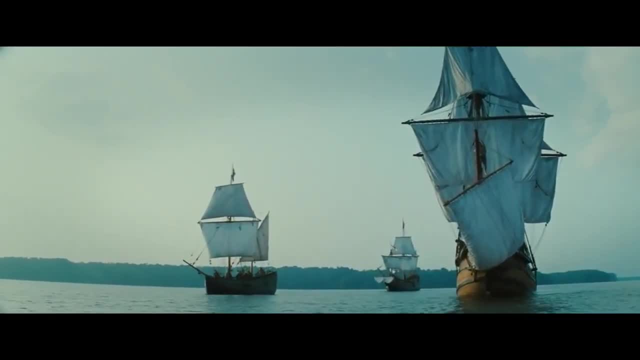 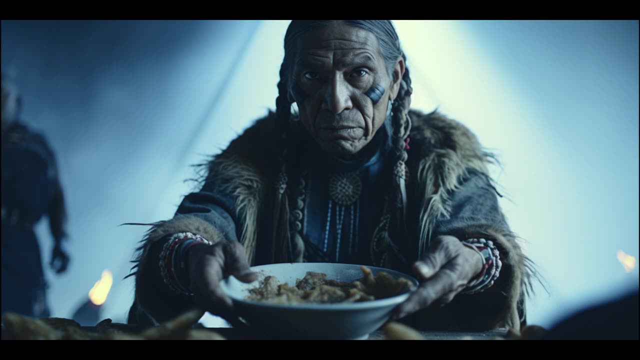 punctuated by the silhouette of English ships. Initially, the English were met with a mixture of fear and intrigue by the native tribes. Despite this, it was early in the 17th century that the English arrived in the United States. Despite this, it was early in the 18th century that the English arrived in the United States. 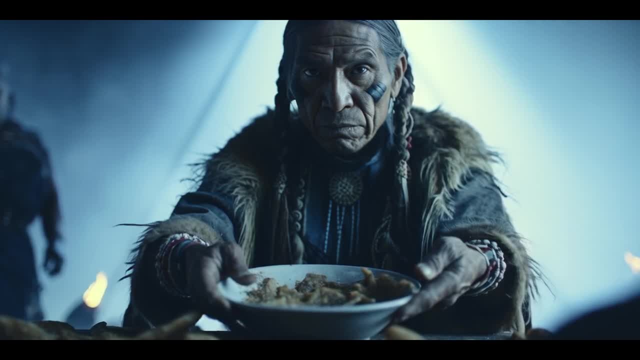 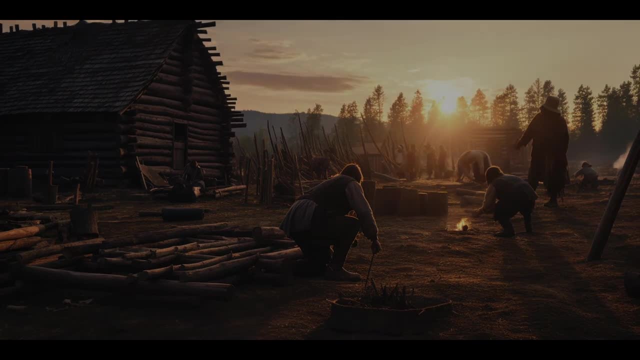 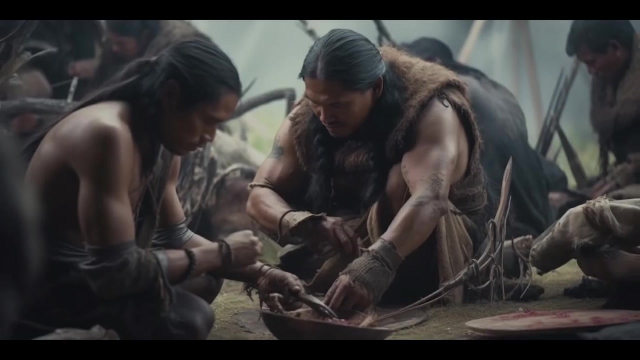 It was the aid from the natives that gave the settlers a fighting chance, enabling them to put down roots and establish the first English settlements on American soil. Trade emerged as the delicate lifeline connecting the New England colonists and the indigenous tribes. This partnership led to the flourishing of local economies. 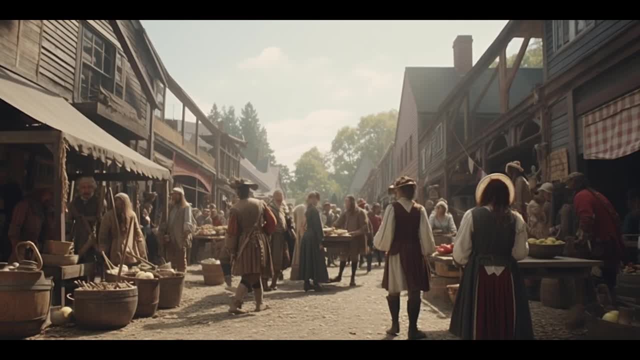 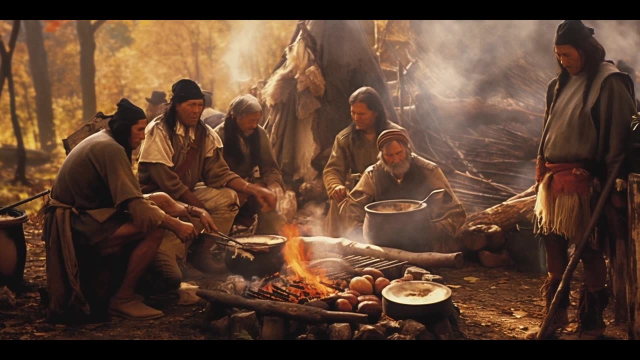 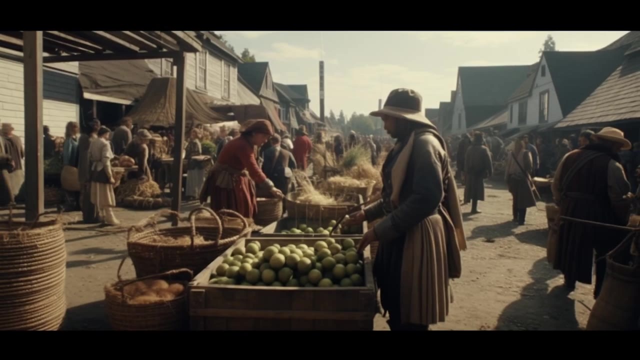 so much so that the Plymouth colonies severed its financial umbilical cord to England within just five years of arriving in America. The settlers and the Native Americans established a distinctive trading system. This system blended the traditions of the Native Americans with the practices of the settlers. 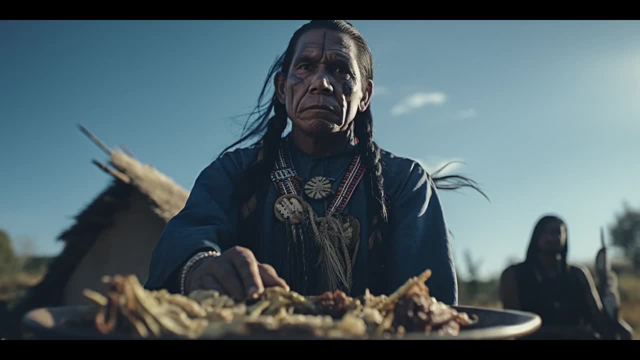 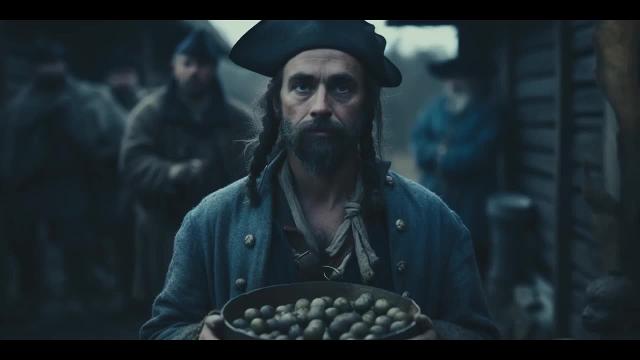 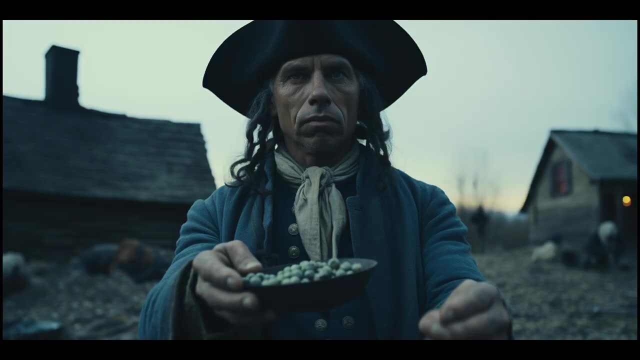 Native Americans supplied a variety of local resources, including animal skins, food and crucial knowledge about the land and its ecosystems. In return, the settlers provided them with beads and wampum, which was a form of currency used by the settlers. However, their exchange 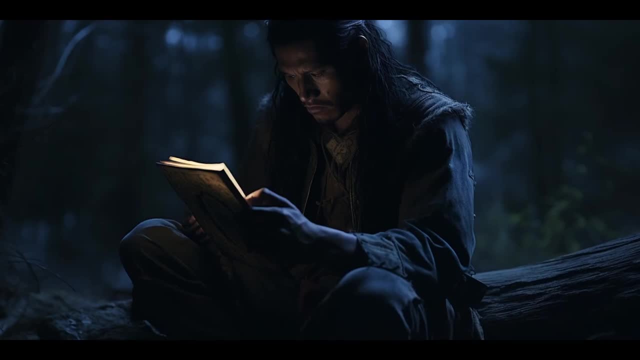 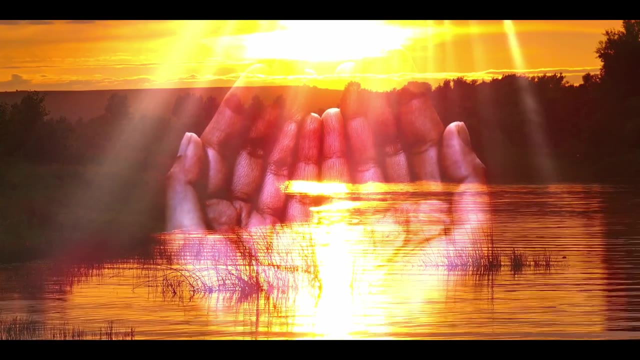 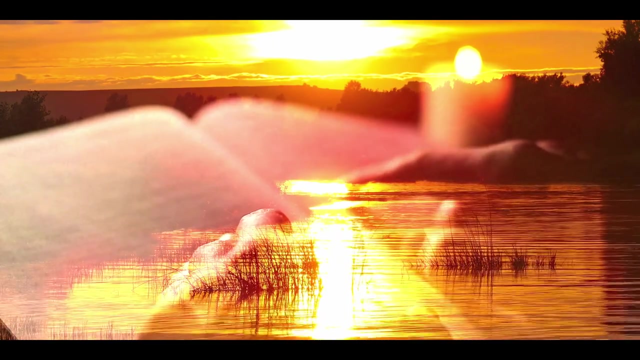 was not only about physical items. There was a significant exchange of ideas as well. In fact, the spiritual conversations between these cultures were so profound that the first Bible in the New World was translated into the language of the Algonquin, a Native American tribe. However, as the sands of time slipped through the hourglass, 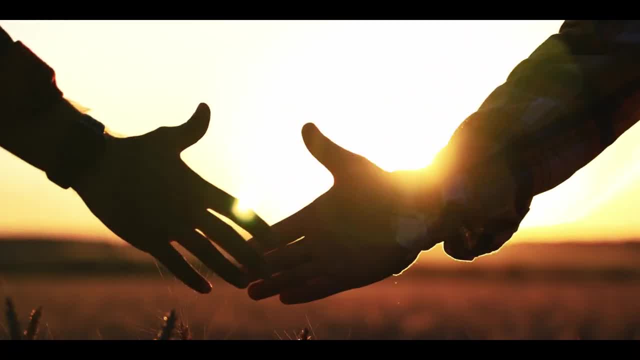 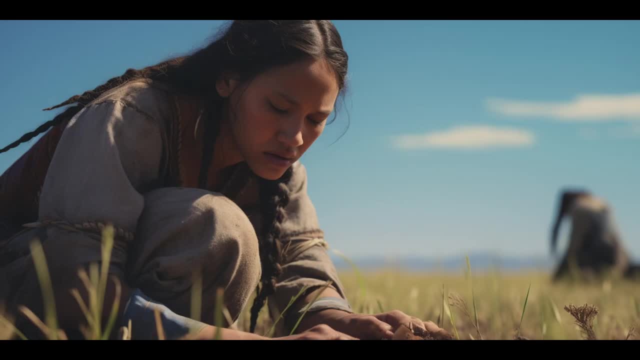 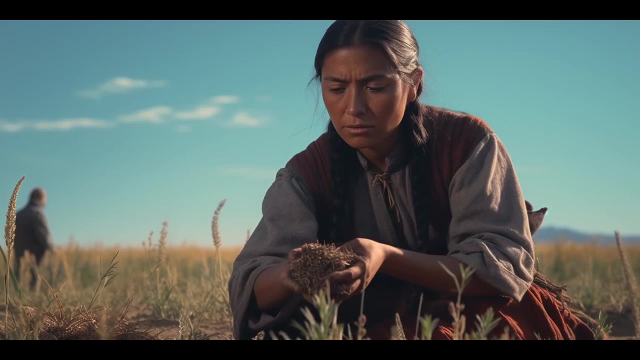 the harmonious relations began to fray. The Native tribes lived by hunting and gathering the abundant resources of the land. Their culture and religion placed them in the role of stewards, not owners, of the lands, preserving its abundance for the future, The white settlers. 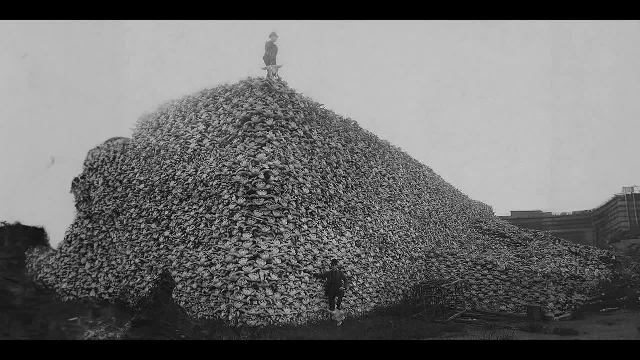 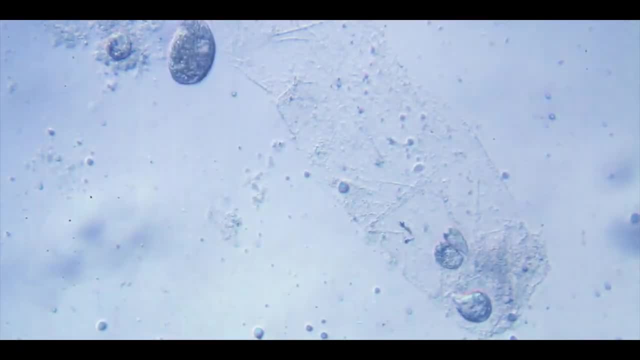 who arrived brought with them a different view of the land. They also brought with them a slew of unfamiliar diseases, such as smallpox, tuberculosis, measles, cholera and the bubonic plague, which all ravaged the native population. The land was then used as a place of refuge for the 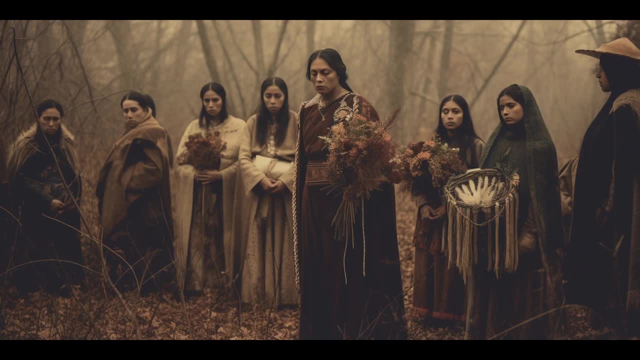 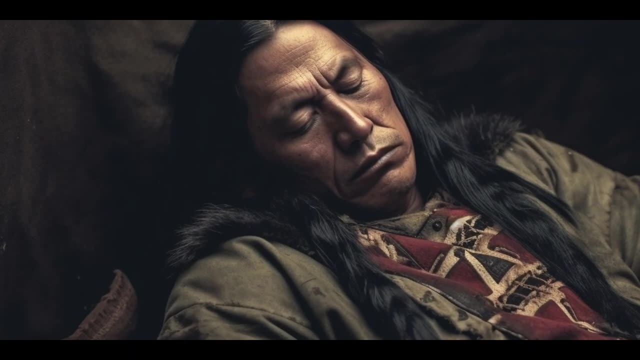 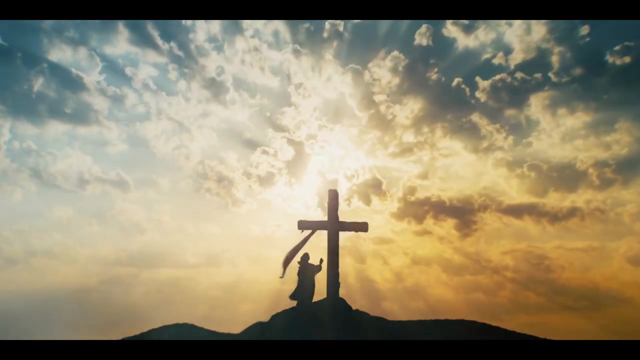 population. This phenomenon, known as the virgin soil effect, led to devastatingly high death rates among Native Americans who lacked immunity to these foreign pathogens. In response to this calamity, colonial governments sought to convert the afflicted natives to Christianity, relocating the newly baptized Praying Indians to Praying Towns. 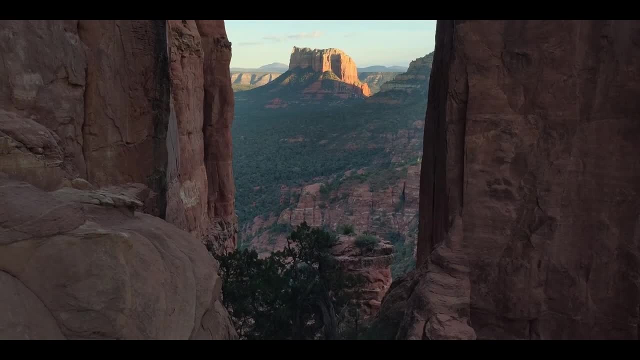 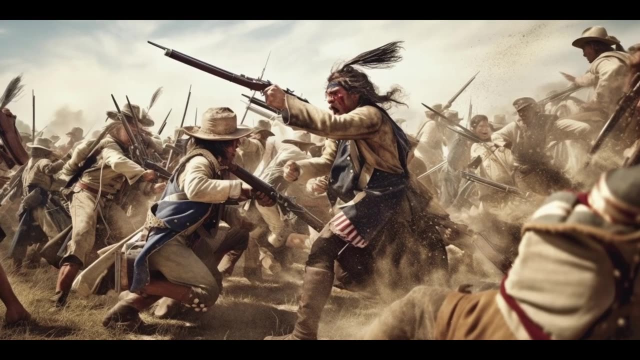 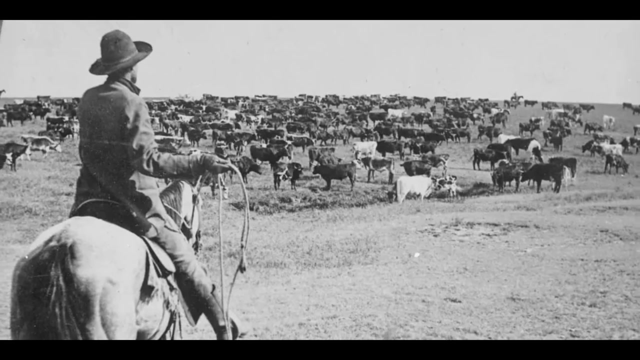 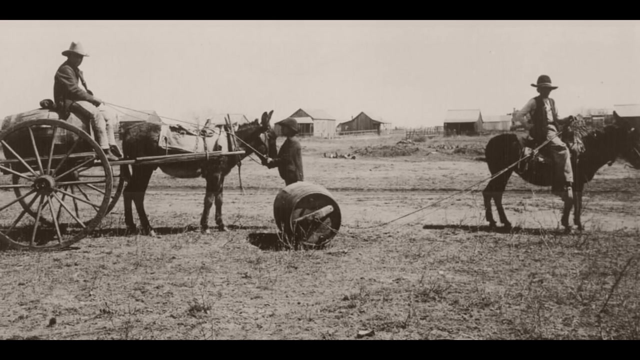 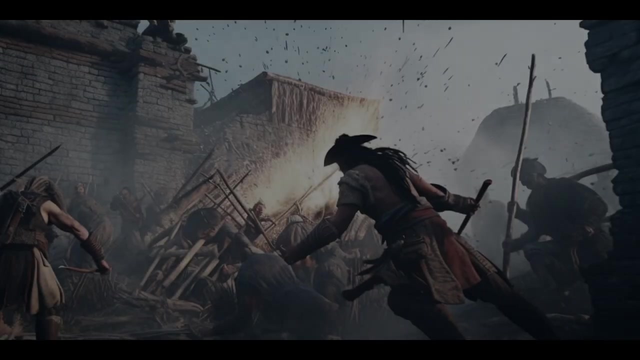 precursors to modern reservations. Tensions eventually erupted into King Philip's War, causing widespread destruction and marking the end of peaceful relations between settlers and natives. The settlers, now known as Americans, managed to carve out a distinct identity from the ashes. The subsequent years saw devastating conflicts between the white Americans and the natives. 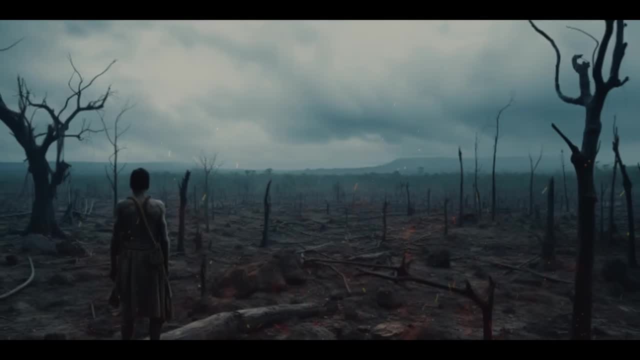 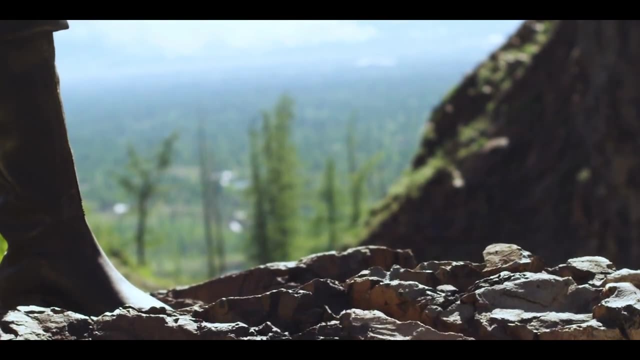 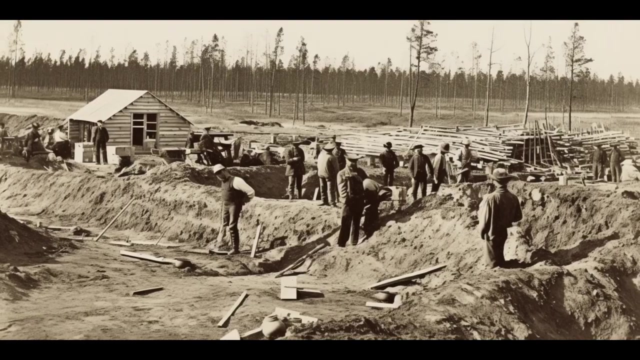 leading to the destruction of more tribes and the loss of more lands. The 1800s gold rush brought even more devastation to the native tribes, bringing white settlers from every place known to man, tearing up the natives' land rights, then overusing the land where gold was found, creating drought and starvation for themselves. 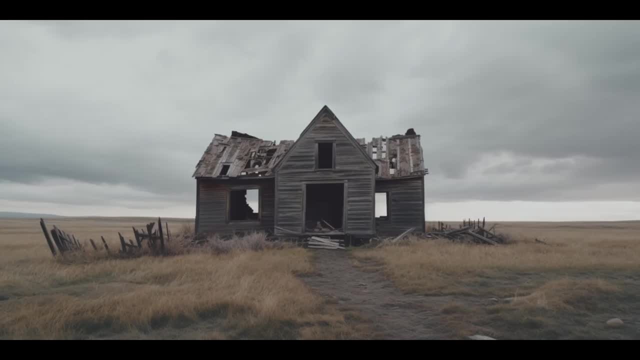 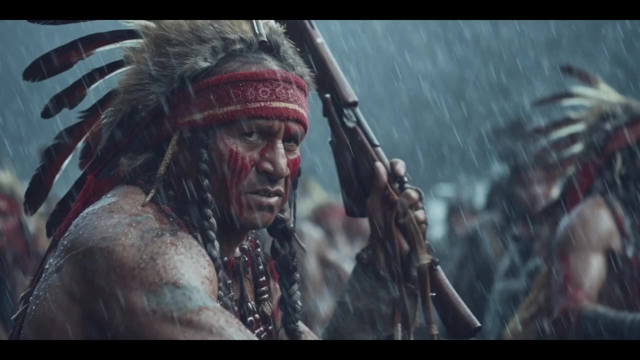 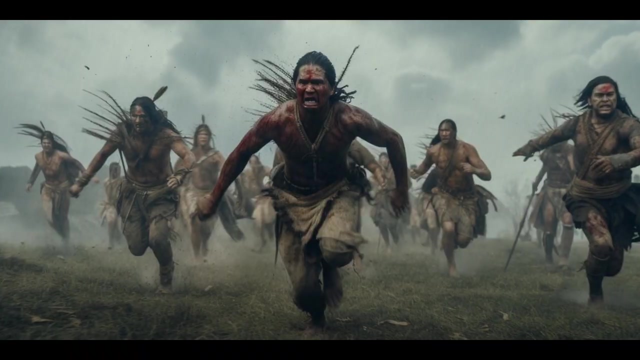 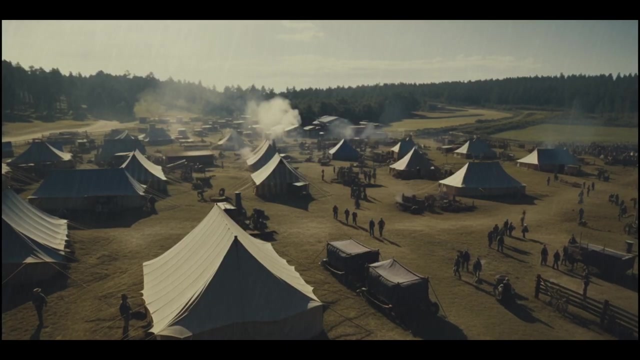 and for the native people, then forcing the natives onto reservations even further from their homes. Despite everything, the natives fought relentlessly to defend their lands and identities, Battle after battle after battle, But their resistance could not overcome the military might and technological superiority of the US Army. 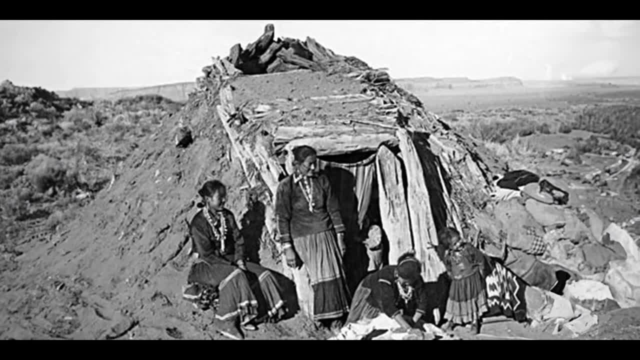 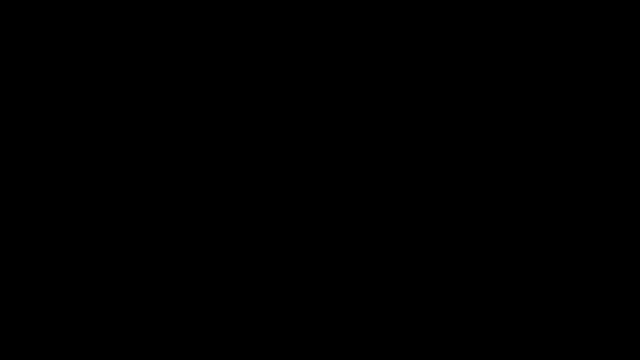 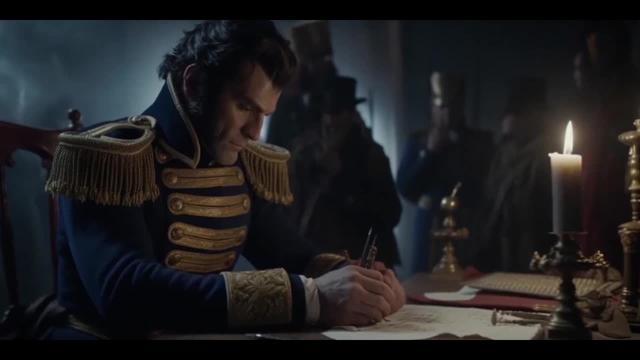 and over time they found themselves exiled to reservations in isolated, inhospitable regions. Throughout this tumultuous period, there were efforts from the settler side to establish peace. Various treaties were signed, peace agreements made and laws passed to protect native lands and 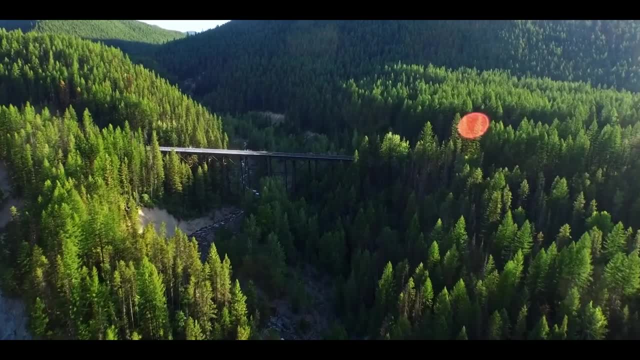 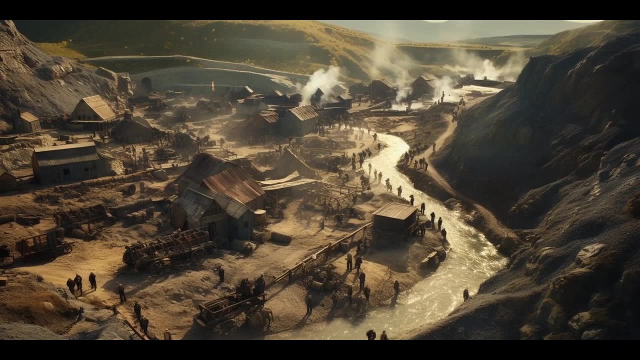 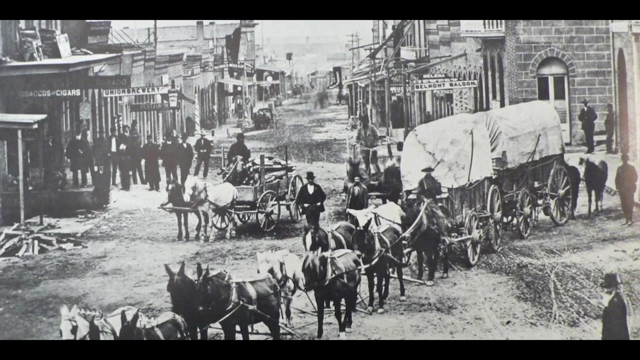 rights. Some settlers even intermarried with natives, blurring the lines between the two cultures. However, these efforts were often undermined by larger forces of expansion and greed. So in the 19th century, while the American population grew by 20 to 30 percent, every 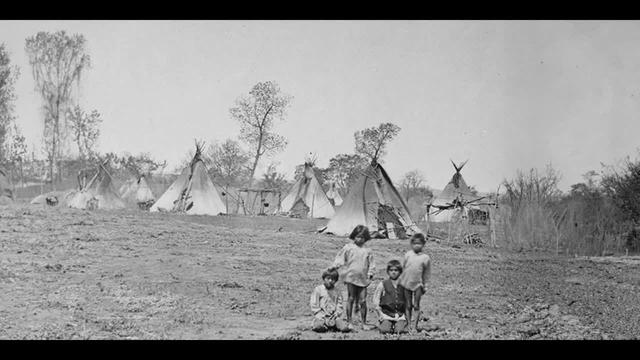 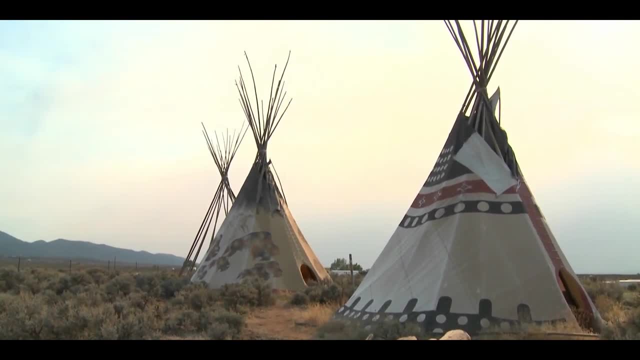 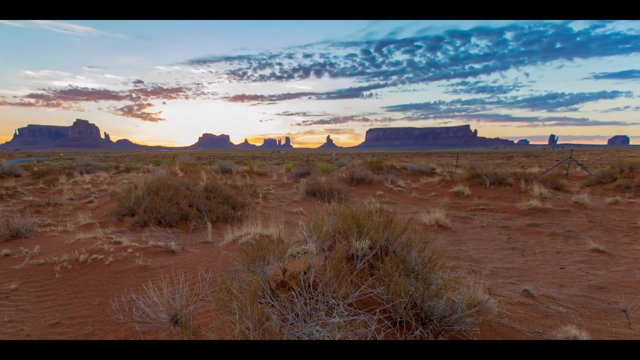 decade, the indigenous population dramatically declined. Today, indigenous and Alaska native peoples represent only 1.3 percent of the total US population. Currently, about 310 Native American reservations scatter across the United States, covering about 2.3 percent of the nation's. 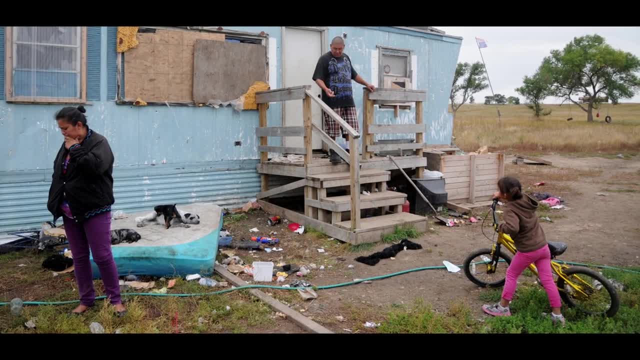 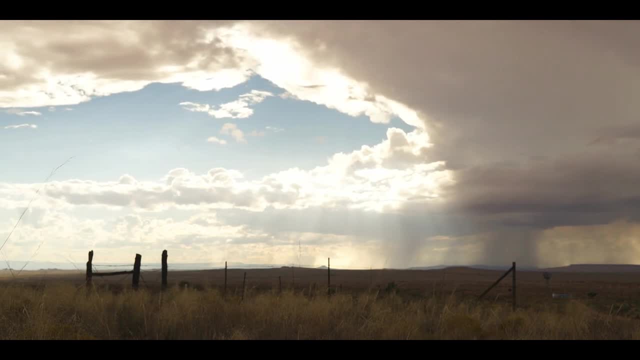 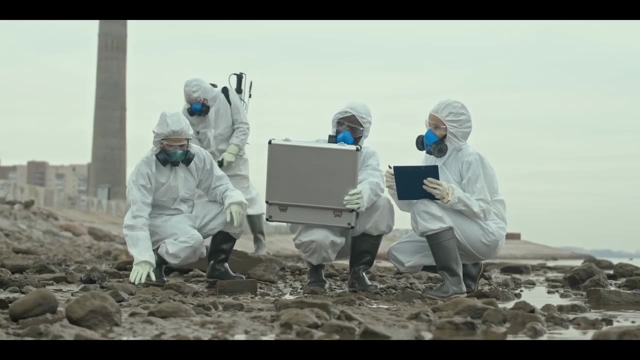 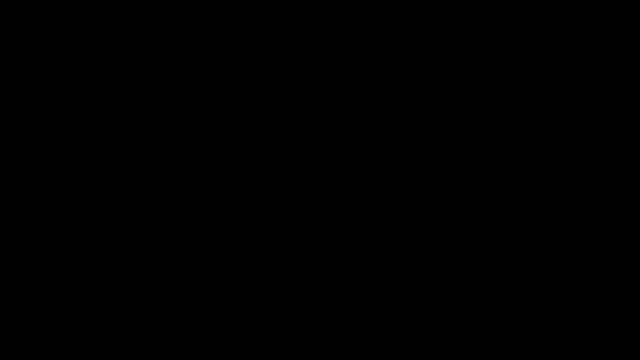 territory. These remote lands offer sub-standard living conditions and limited access to vital resources. Due to lax environmental and health regulations on reservations, native tribes are frequently exposed to significant amounts of radioactive and other hazardous waste. This leads to cancer rates much higher than the rest of the country. Despite no longer being the targets of 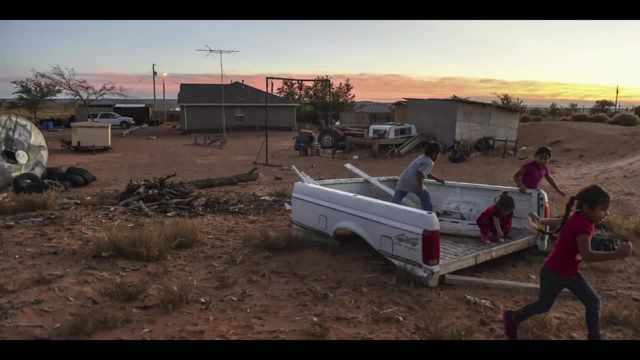 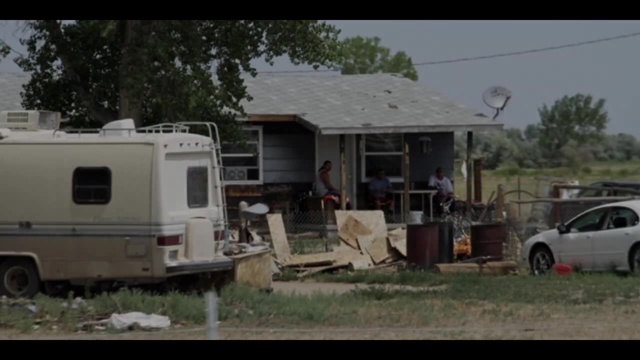 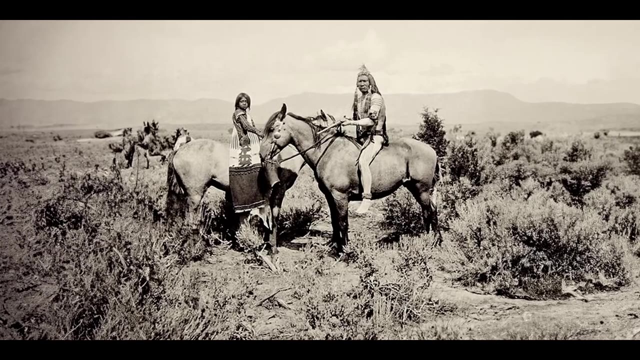 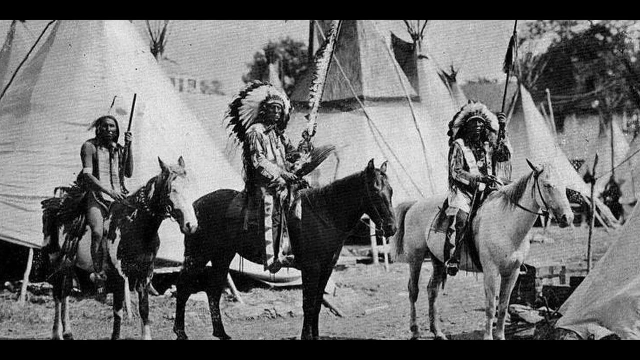 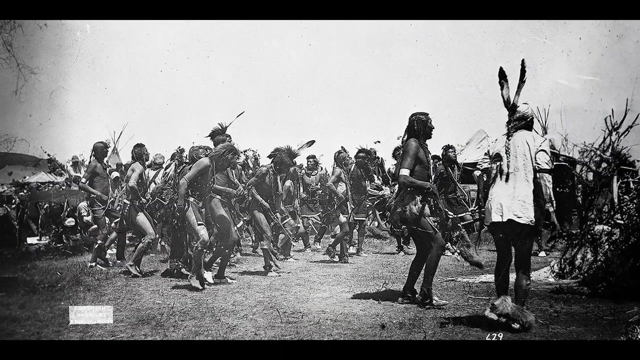 extermination. indigenous peoples figure out how to protect their lands and territories. The past echoes the present, and the future is shaped by its own indomitability. The land of the Native people is a place of ignorance, invisibility and discrimination. But remember, it wasn't always this way. There was a time when five million natives roamed the plains, living as one with nature. and though the plains may have changed, their spirit endures A testament to a past that echoes into the present, shaping the future in its own indomitability. 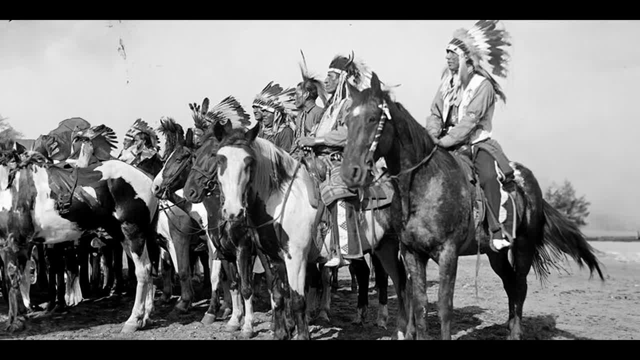 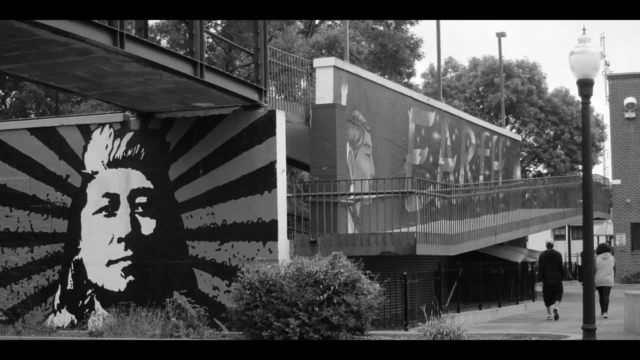 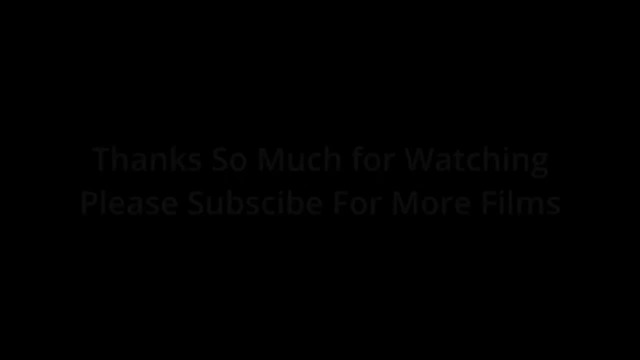 The song of the plains is not forgotten. It reverberates through the ages, sung by those who remember, those who honor and those who dream, laughing lalala, la, la la﹐ Herts. screenshots are hard. low or low, oh. amazing. you myös resonate with you, 涼.